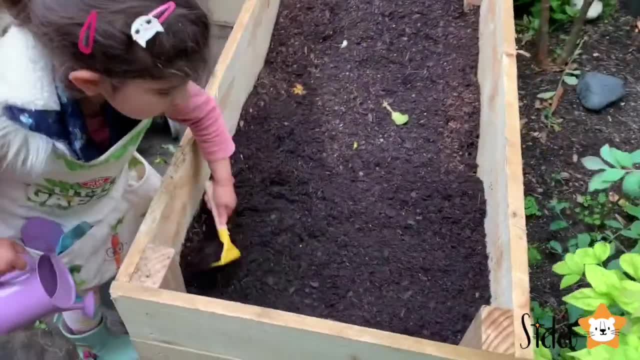 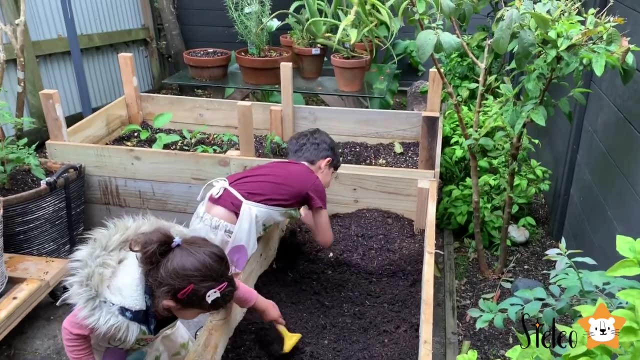 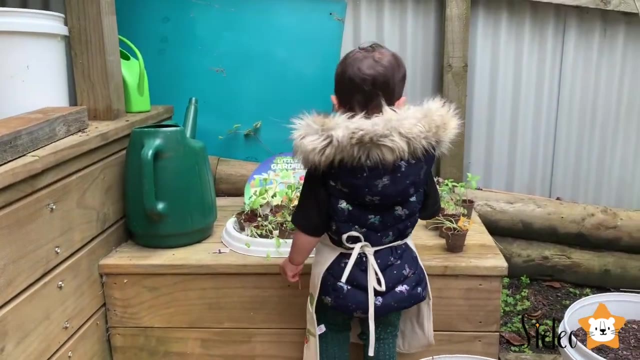 Okay. so Leo and Stella are straightening the soil up- Well done, Okay- with their little racks. Okay, what is Zaza doing? This is what you're doing. Yeah, Yeah, Come here. Finished guys. All right, it's finished. 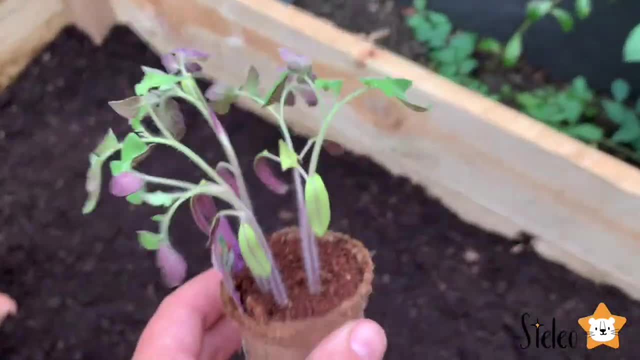 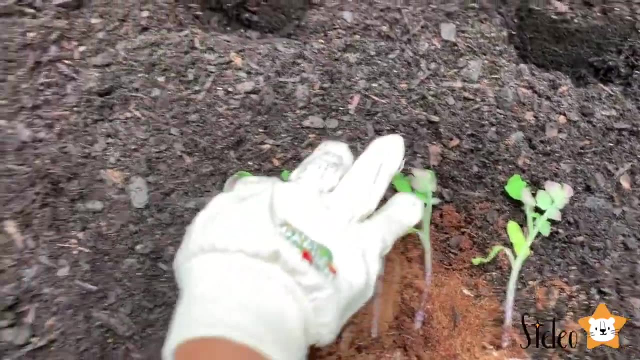 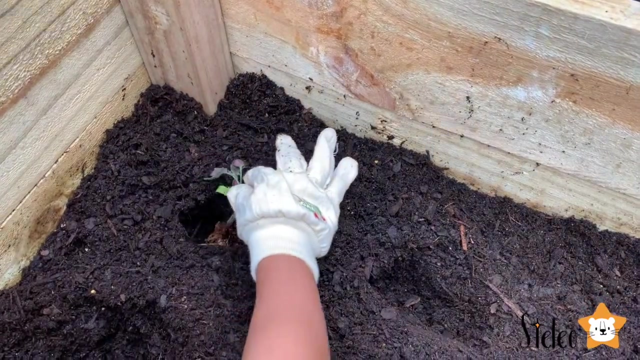 Are we ready to plant? Okay, you want to take one Carefully and put it in the first one. Put it in Nice, Nice, Hold it, and with your other hand you cover it up. I'll hold it like this and you put the soil. 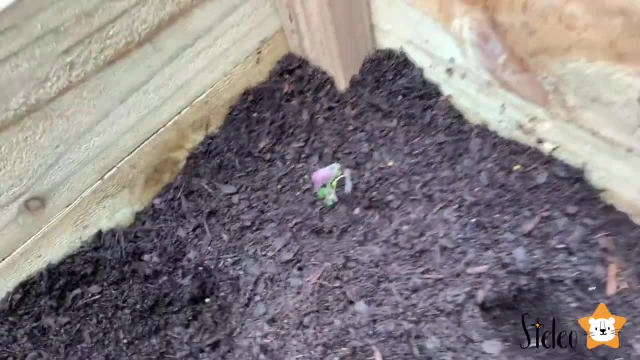 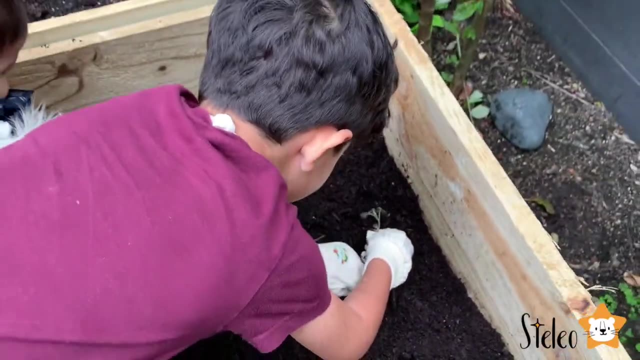 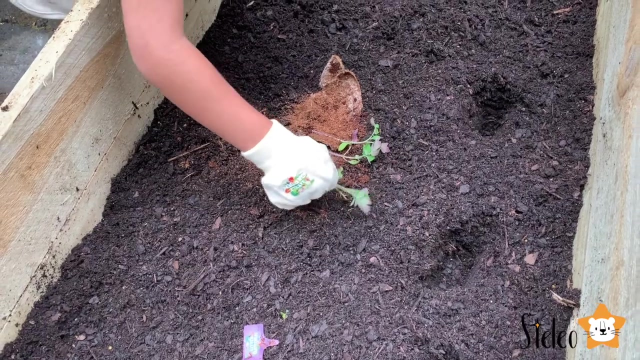 Now, Now, Ready, Woo, Okay, Can I do the other one? Do you want me to hold it? No, I got it. You got it. Well done, I love this. Yeah, Yeah, Hold with one hand. 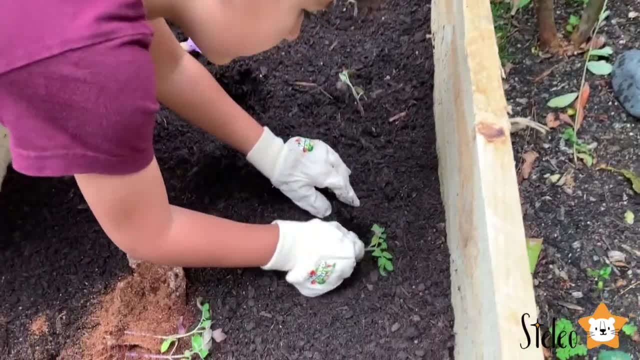 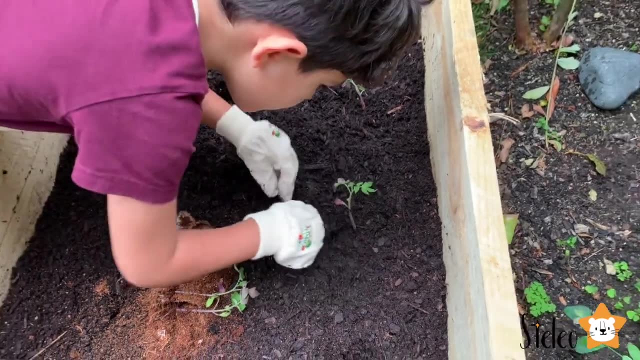 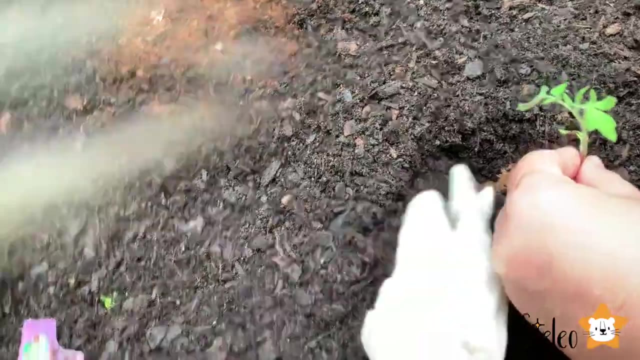 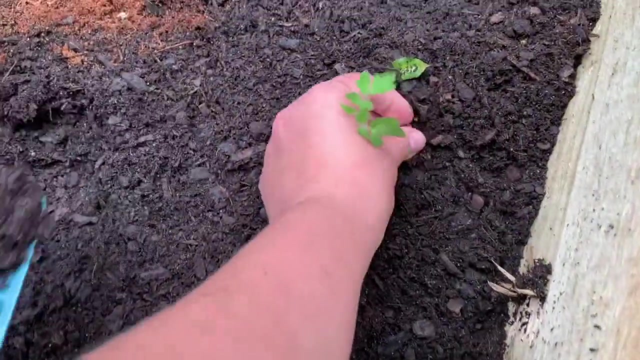 Wait, Okay, My turn. Oh, it's swimming. Look at the roots. Well done, Stella. I know This is my trouble, Yeah, But not on the plant Near the plant, Okay, Just near the plant. Where's Stella? 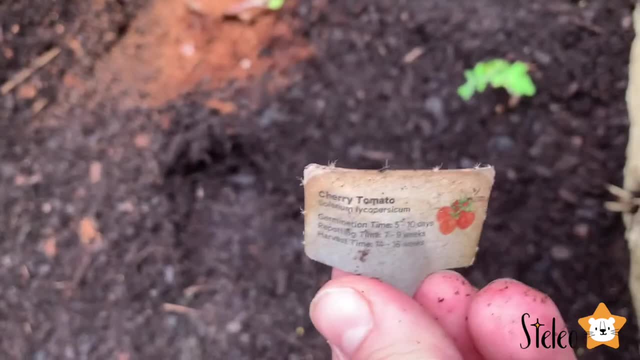 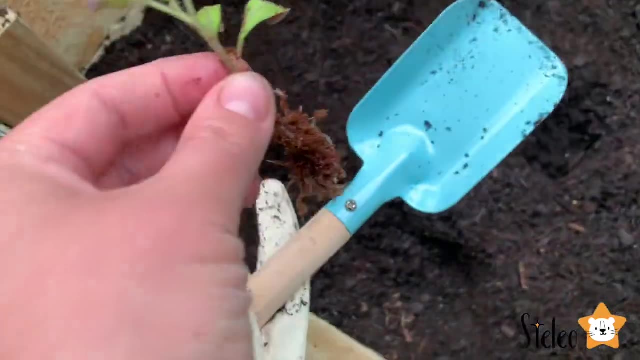 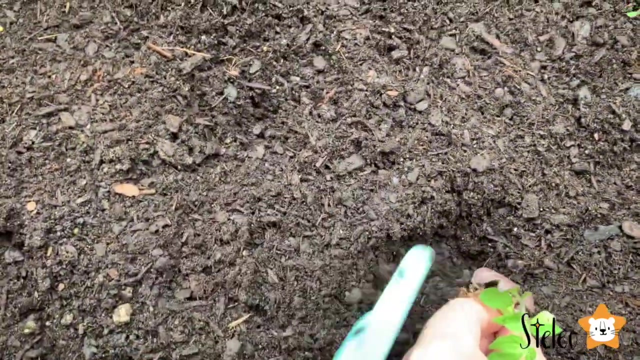 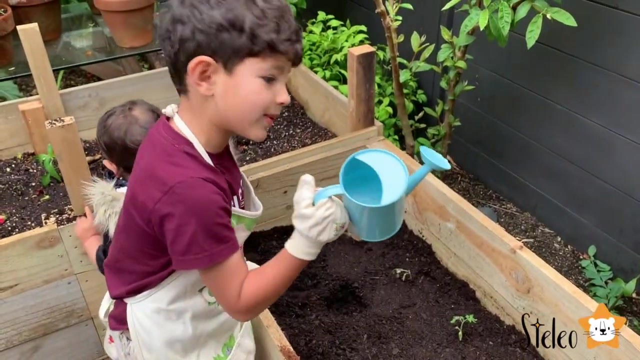 And this is cherry tomato, Stella's favorite, Not really my favorite. Let's do it. Oh sorry, I'll hold it and you cover it. Yeah, Well done, Guys. now it's time to go. Let's go. 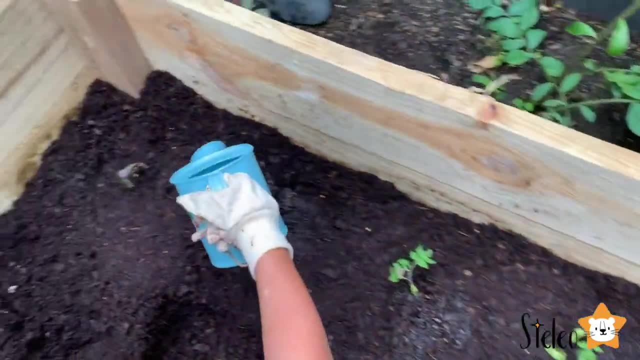 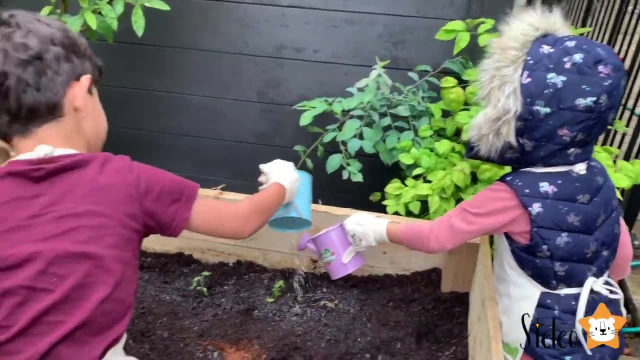 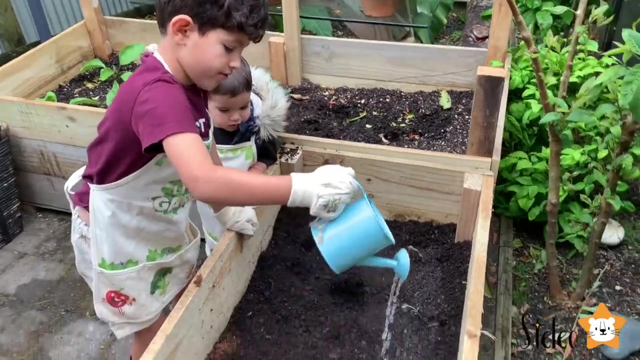 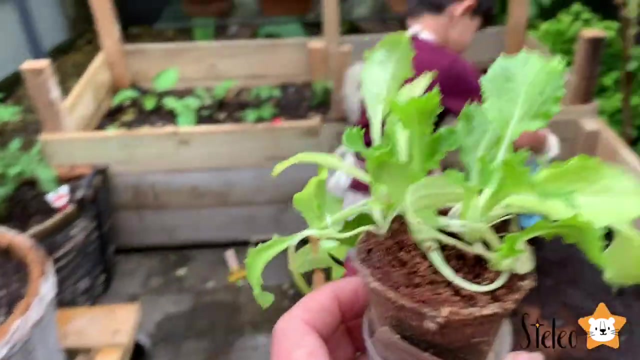 Oh, well done. Look at one of Stella's claws. Are they supposed to fall? Very nice, well done. What should we plant next? Are we ready for the lettuce? Yes, Yes. Are you ready for the lettuce? No, 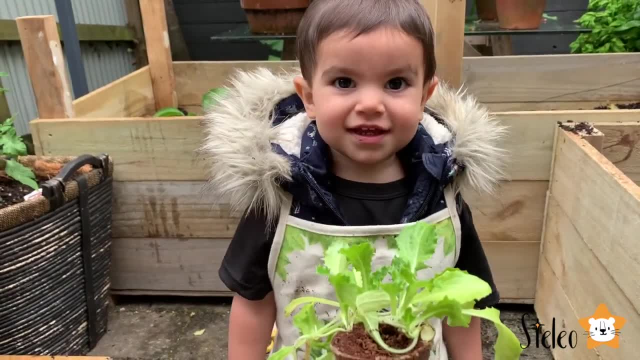 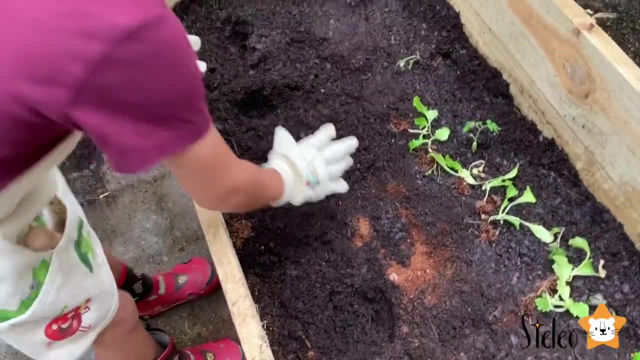 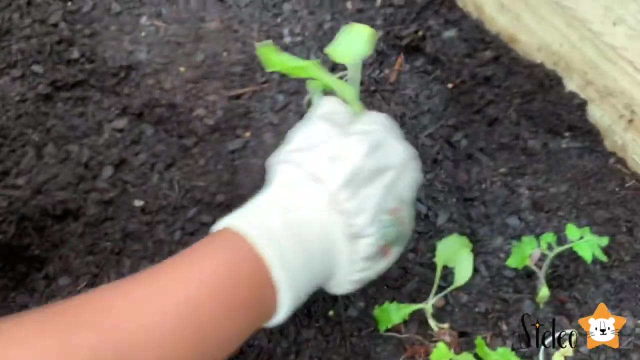 Nope, Do you want to do the lettuce? Okay, let's do the lettuce. Now we have to fold it and cover it. Yes, I'll get the fold. That's all ready. Yeah, We're going to get a lettuce. 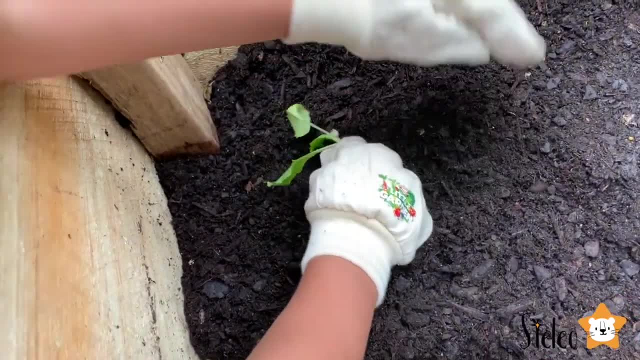 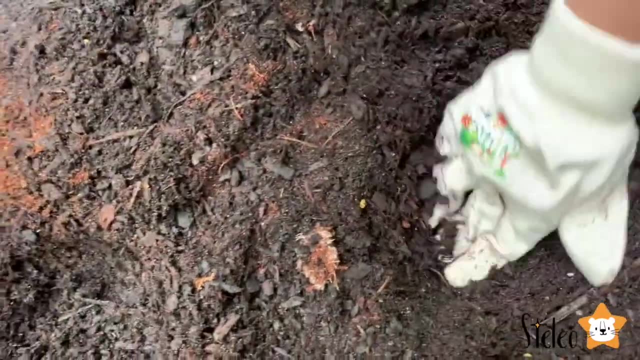 And we're going to cover it with foil. Well done, And then I'll do it. Yeah, You want to put two of this here? Come, Take one lettuce. Okay, Stella, Just put it here and then cover it with foil. 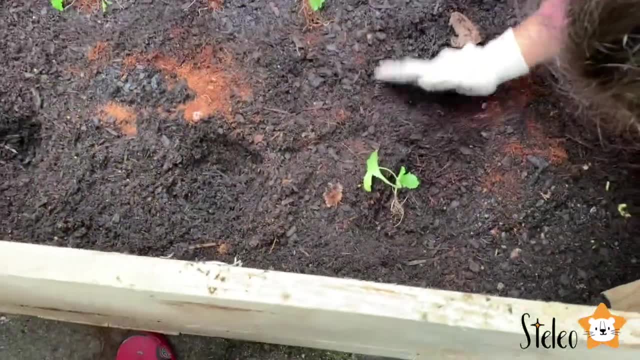 Finished, That's all done, and now we're ready to water them. Mama, if you put too much water, it's not going to work. Yeah, but now. Oh my God, Oh my God, Oh my God. 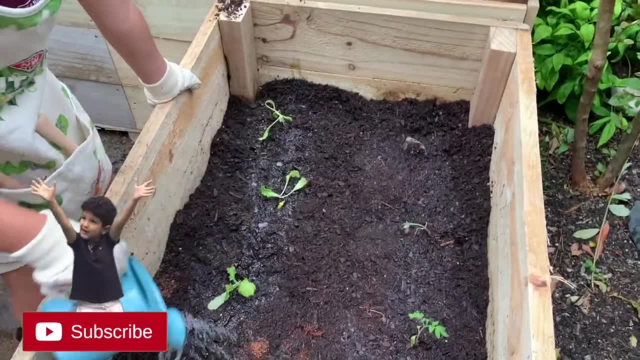 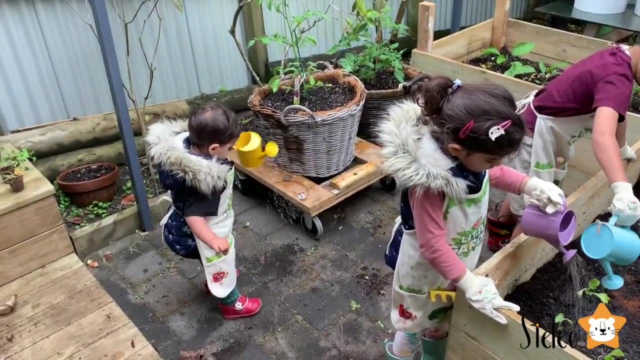 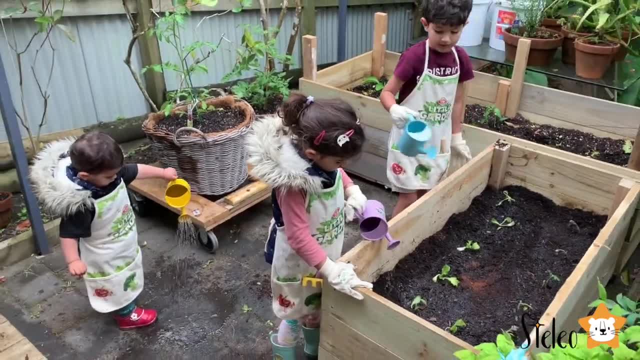 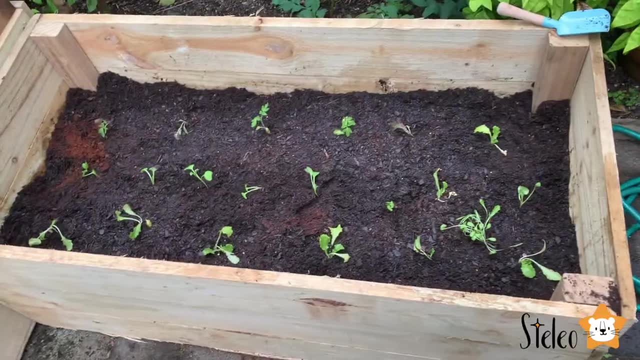 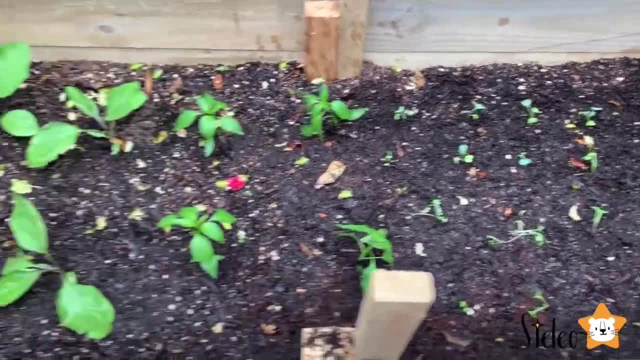 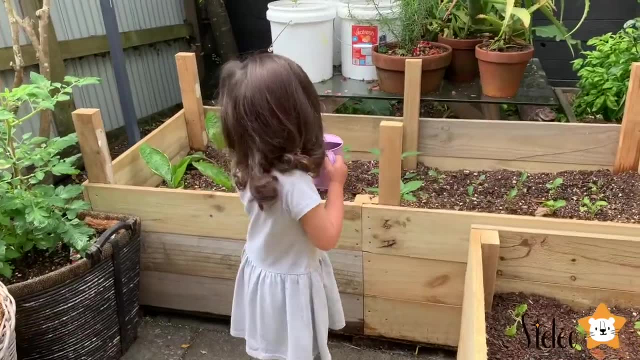 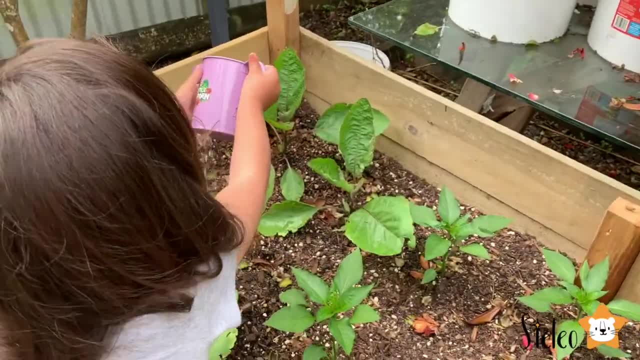 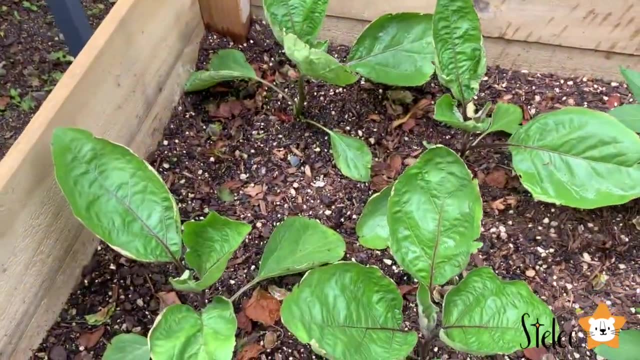 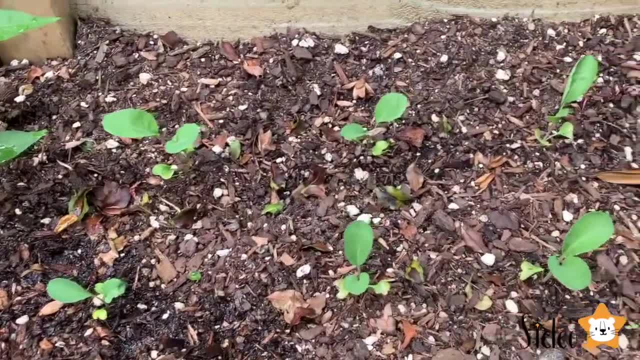 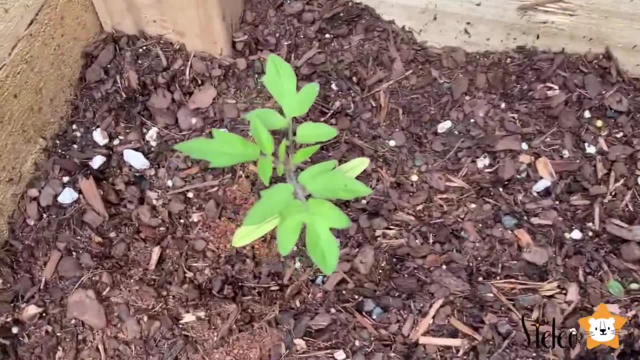 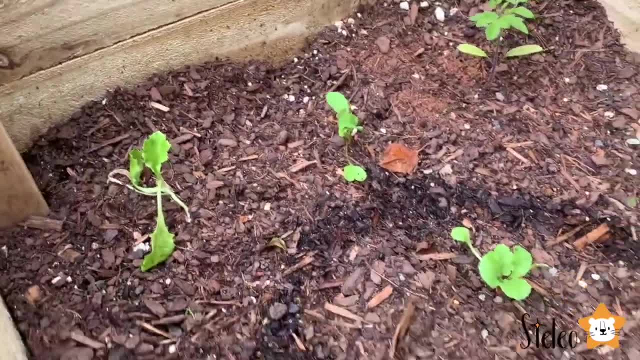 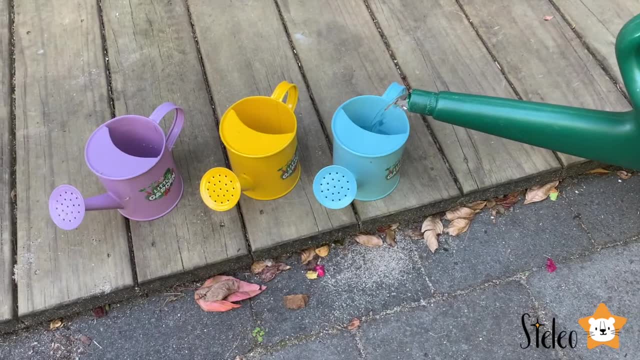 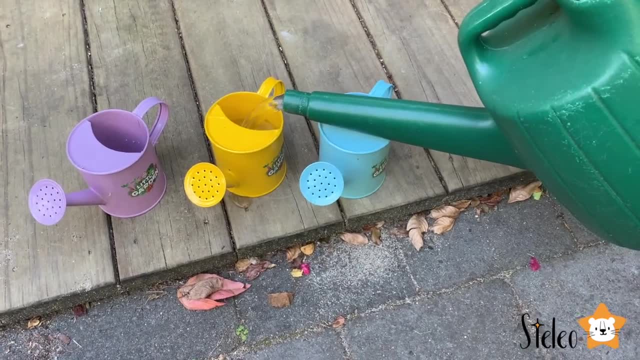 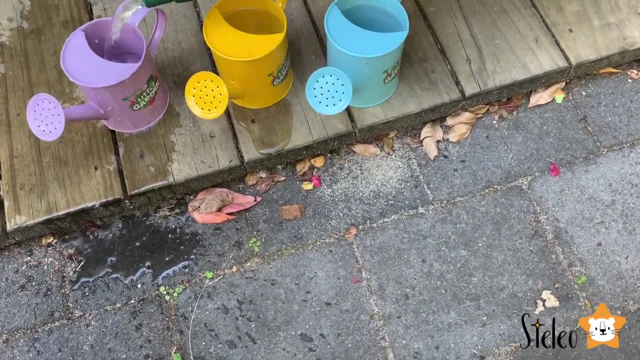 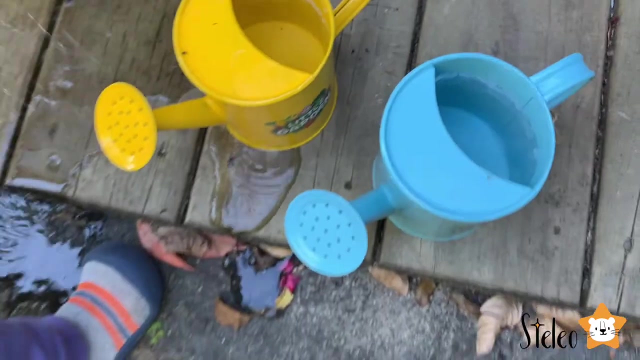 job in one bus. I remember eating my meal in my RV and I remember running pretty disheveled. today, I And the last one. Whose is this? Okay? whose is this one? Alright, Okay, now we're gonna water. Leo, can you take him? 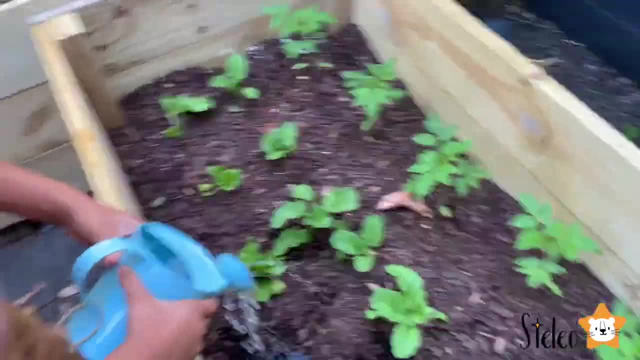 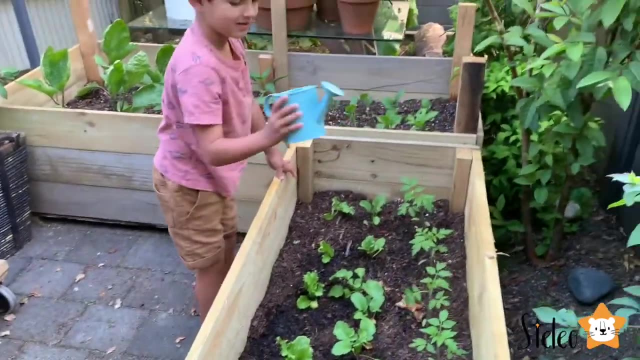 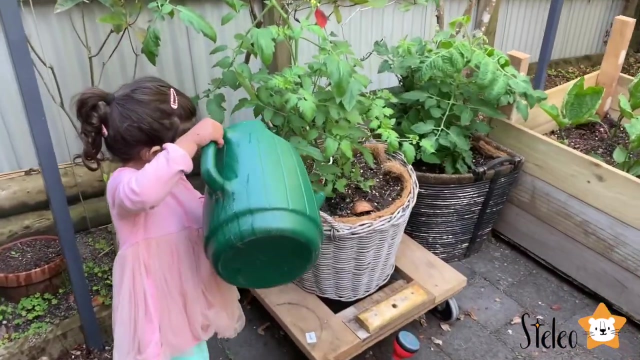 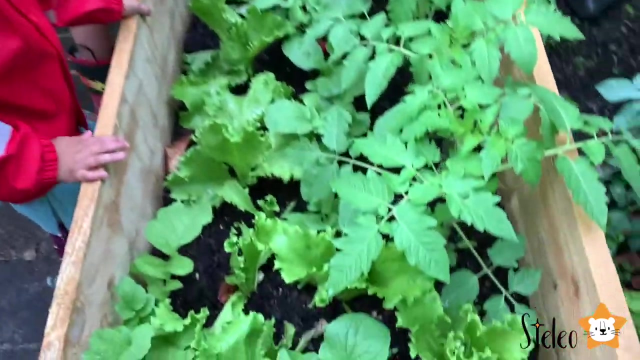 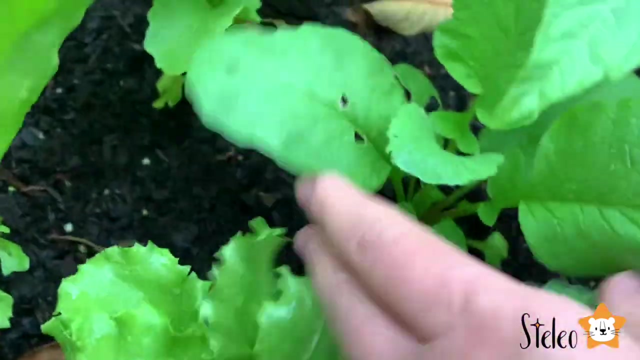 Oh no, goddamn, Let's water Leo, Hello, Wow, The big one, Wow, and look at those big tomatoes. What? And there's even one right there. Oh, my goodness, look at this. Look, there's the radish. Wow, shall we pull it out? 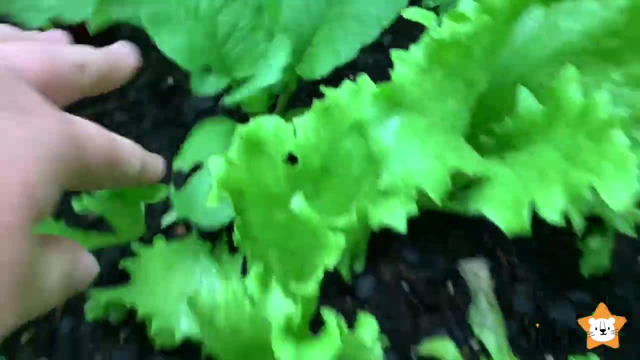 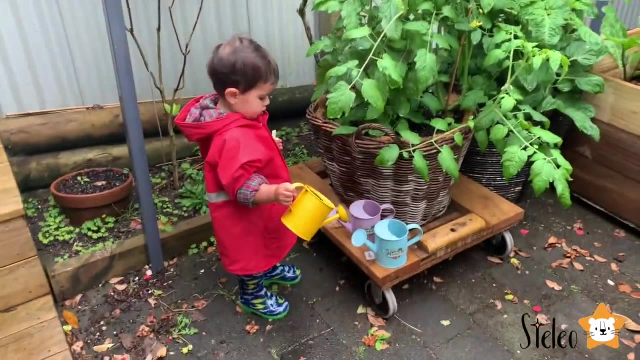 I think we're gonna let them grow a little bit more. And look at this lettuce. How do you think one of them is here and one of them is here, And you know all of them are good. Okay, which one do you think is the biggest? That one. 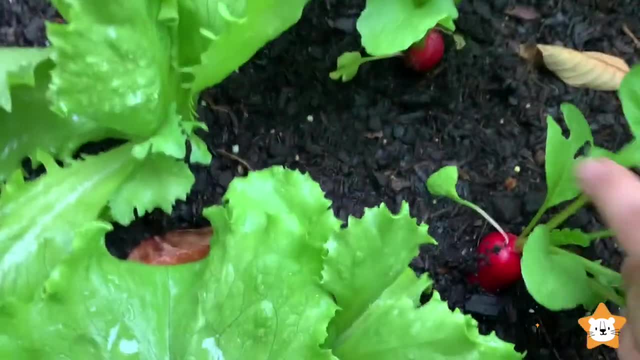 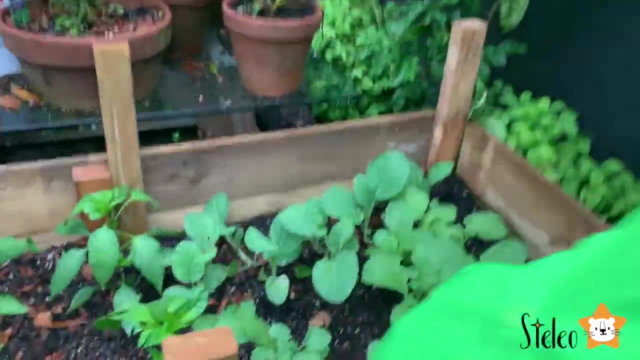 This one? Do you think it's the biggest? I think this one is the biggest too. Yeah, I think this one is also. I think, to be honest, we just have to cover them with more soil. What? Look here, Leo, Look wow. 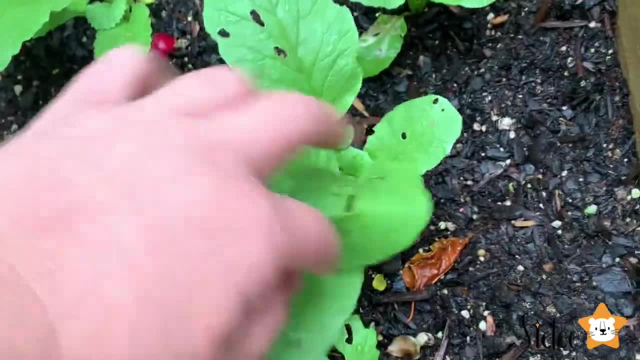 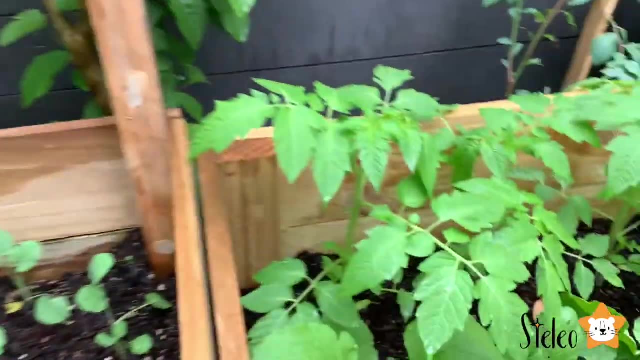 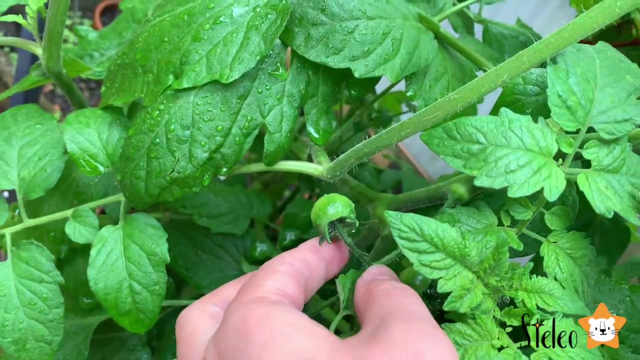 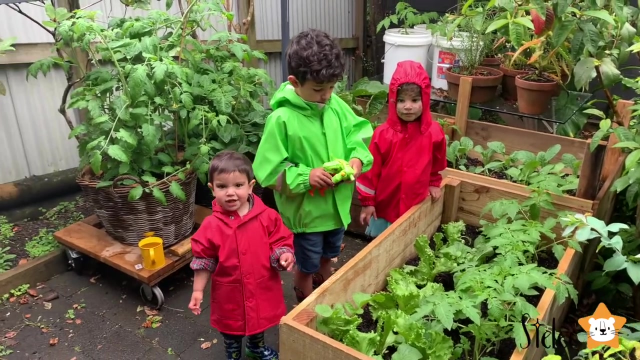 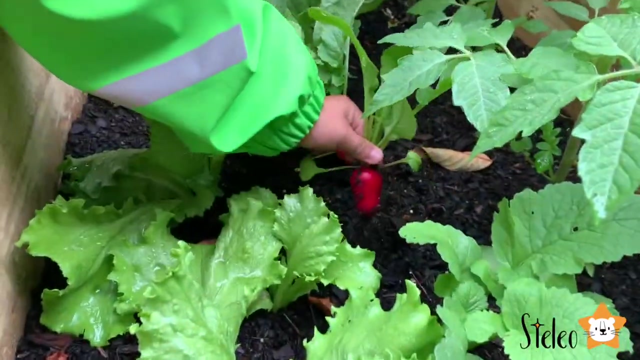 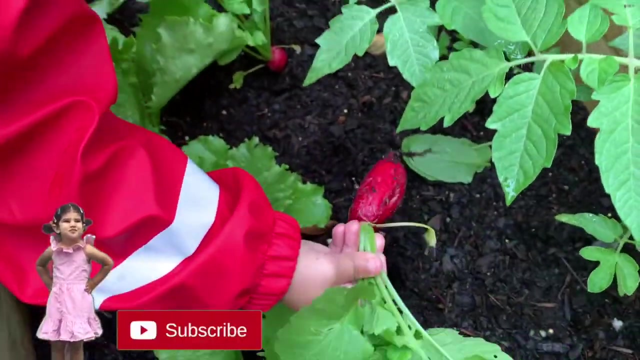 Look, I think we're gonna cover them with more soil and tomorrow they're gonna be ready to Tomatoes. Oh, look at these tomatoes. they are ginormous. They're so big Cheese Guys. now we are going to pick one. Oh, look at this. 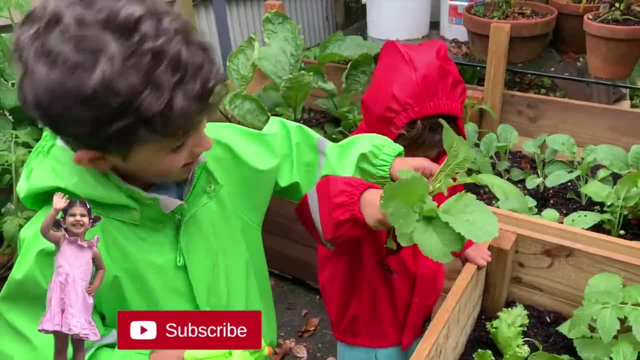 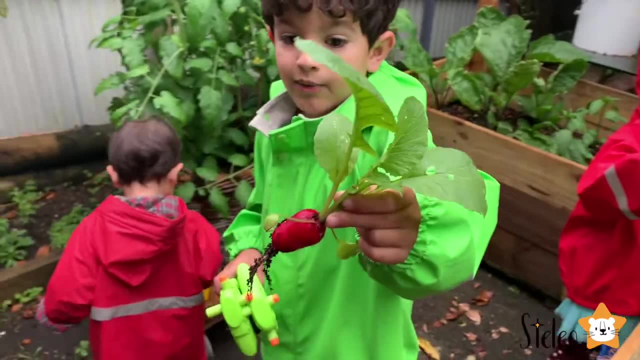 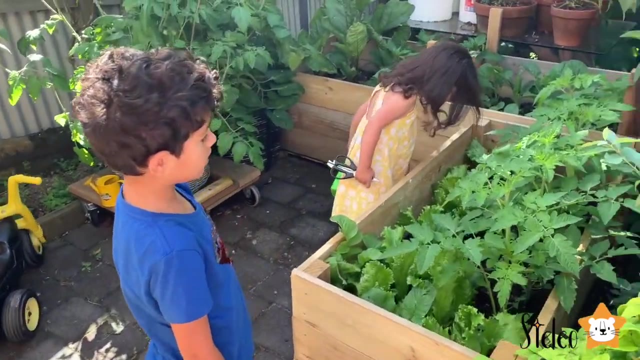 Let's see who is the biggest Sausage. Is it a sausage? Look at this Sausage. Let's see how bad they grow, What It grows- so big Did it grow? Oh my goodness. Look at the tomatoes- ginormous. I can see the radish. 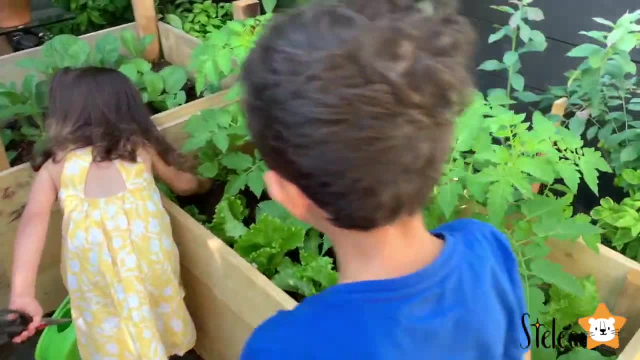 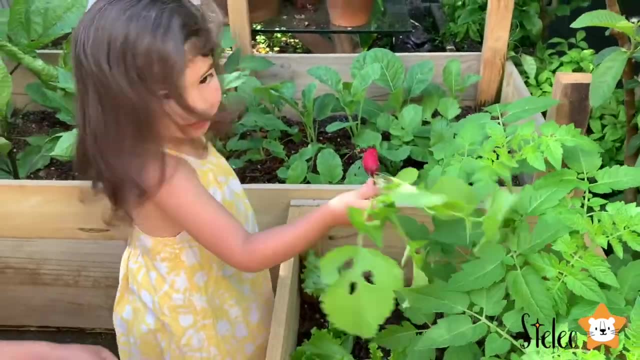 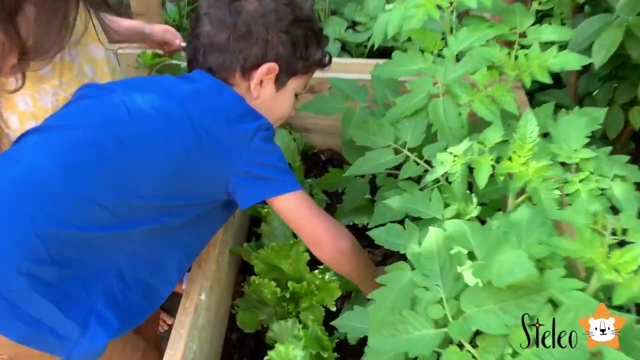 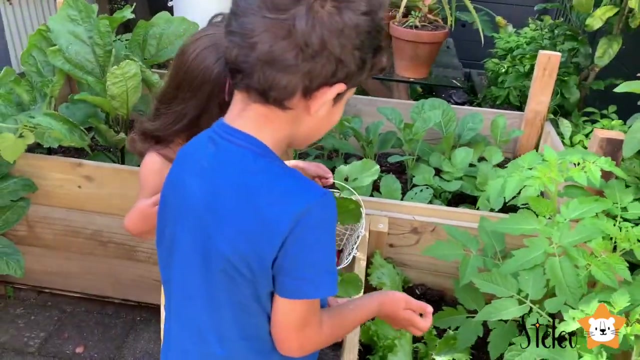 Where is the radish? Last one: Okay, give me those scissors. Look what? Okay, do we want to put it in the basket? Hello Zaz, what are you doing Now? this is spicy, Oh, wow, It's spicy Now you. 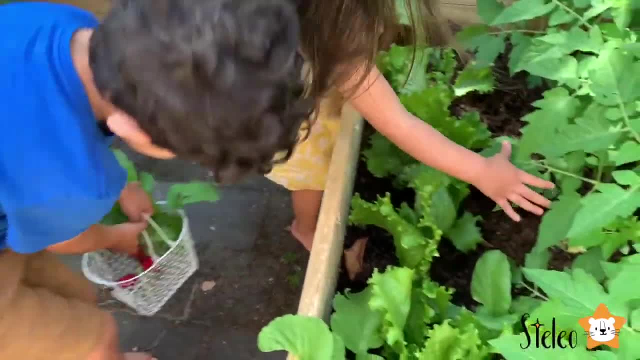 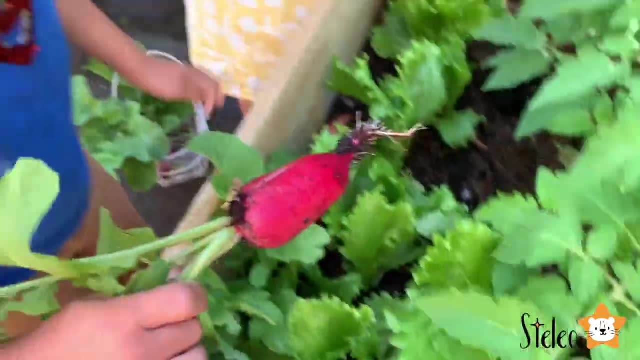 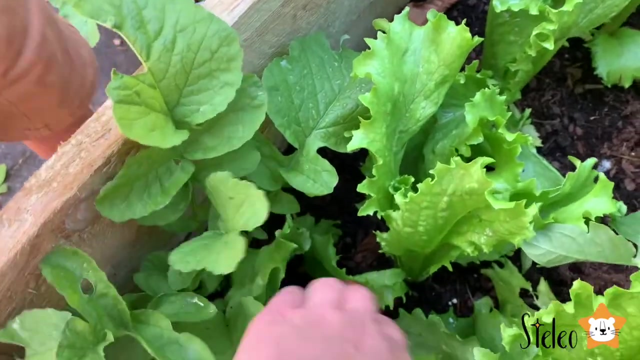 Now you get it. What about this one, guys? What about this one, guys? It looks so thick. It looks so thick. Look, it doesn't matter. Okay, Is there any radish left here? Nope, What about this one? So much radish. 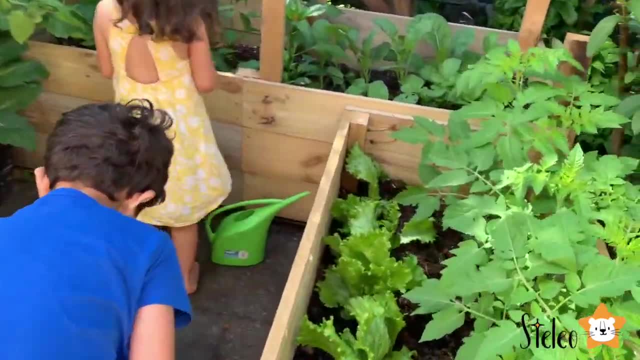 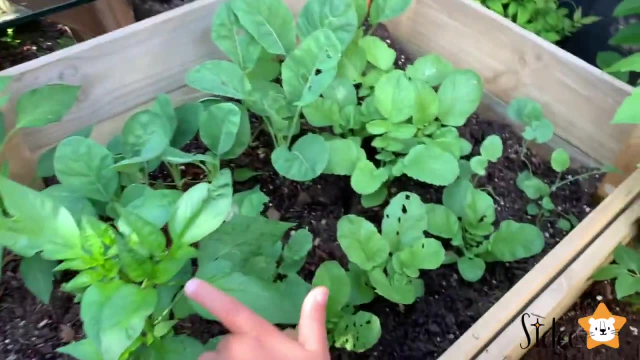 Perfect. I think we've got some radish on the outside. I think we've got some radish on the outside. Do we have some there? Nope, So all of this is radish. Leo. Yeah, found one, Found one. this one's good. 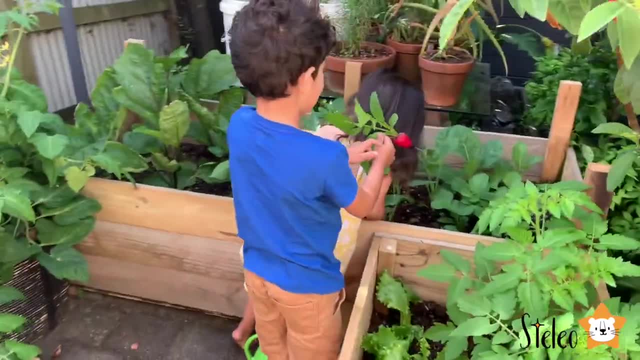 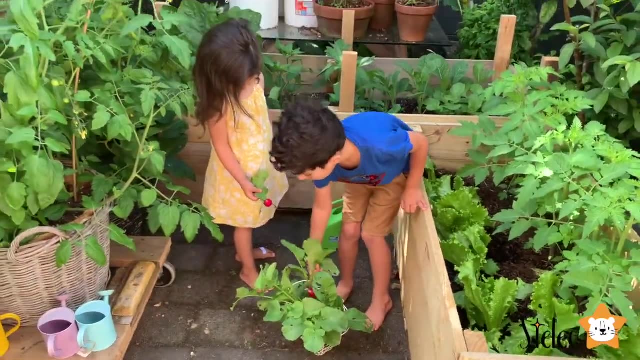 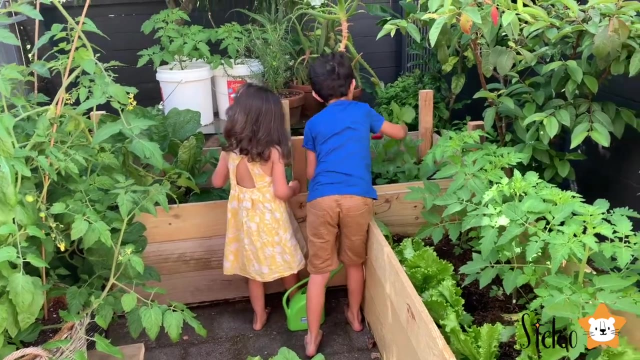 Let me see. let me see We have caterpillars. Can you see it's bunched. Can I see? Look it's bunched. All of them are good. So you know now which is the radish right. Look at this one. 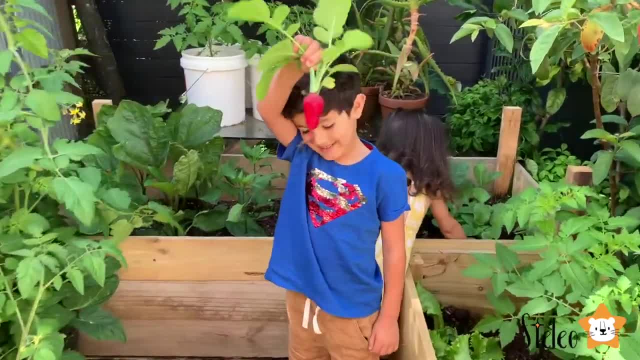 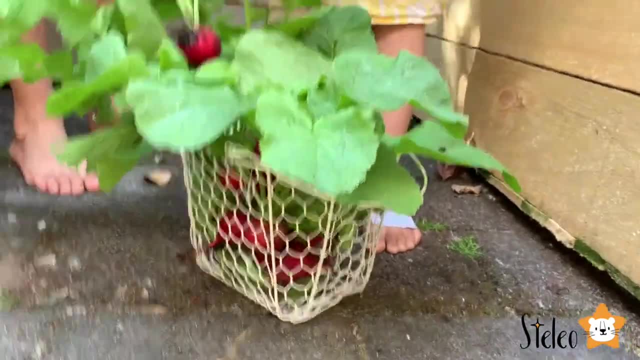 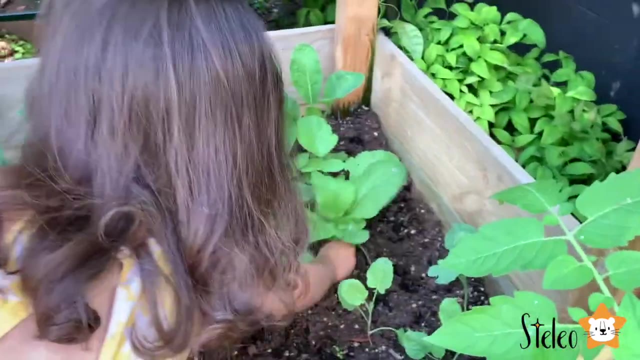 What? But look how good it is Very nice. oh, my goodness, this is going to make Salad, It's going to be salad, It's going to be salad, It's going to be salad. A little bit more, A little bit more. Mama, is this radish? 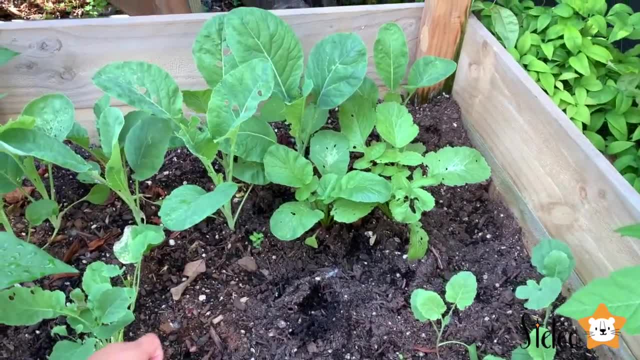 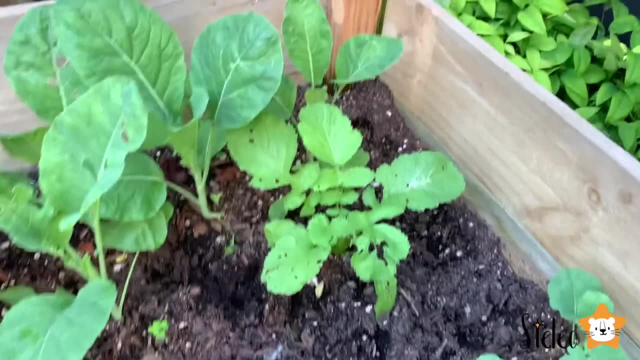 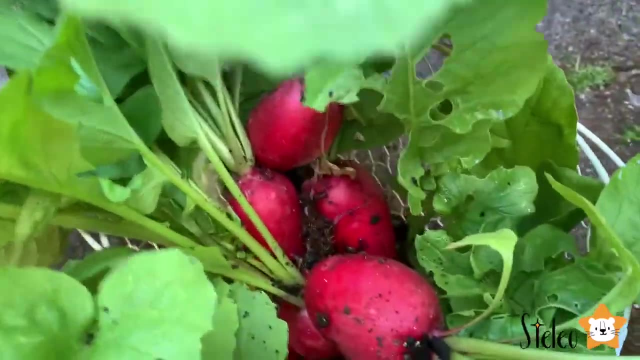 Mama, is this radish? No, but the one next to it is radish. No, but the one next to it is radish. Oh, I just see the radish. So there is one more thing. So there is one more thing. Do you think we've got enough for a salad here? 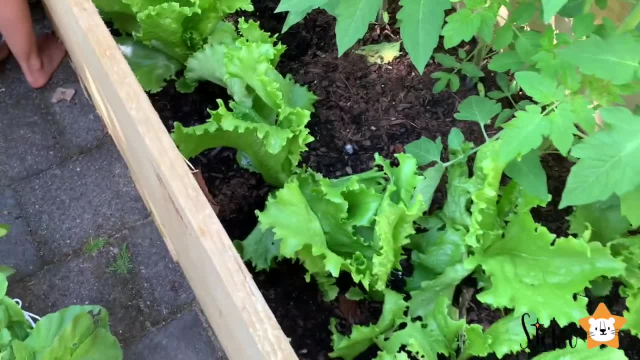 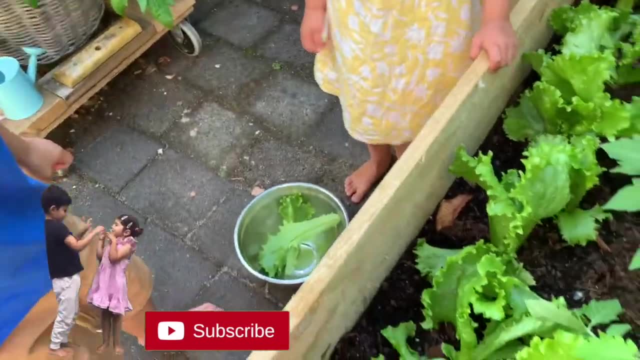 Do you think we've got enough for a salad here, But we have to get some lettuce. Yeah, we have to get some lettuce. Shall we do some burgers. Shall we do some burgers. Yeah, because we have too much lettuce to only make a salad. 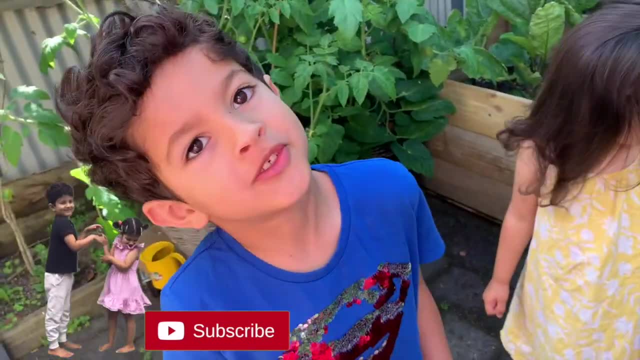 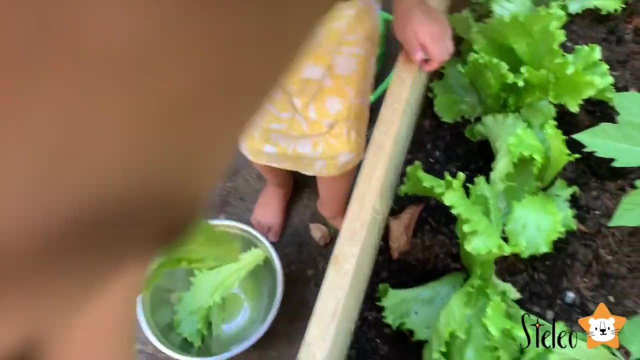 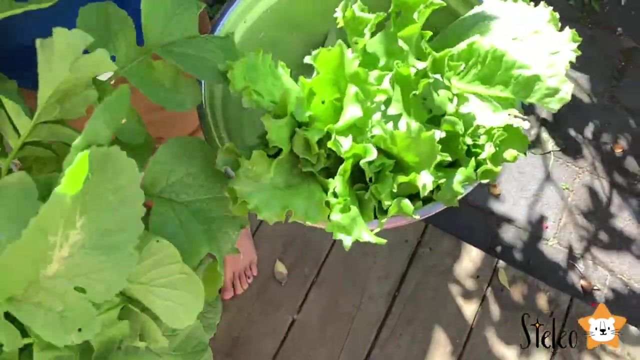 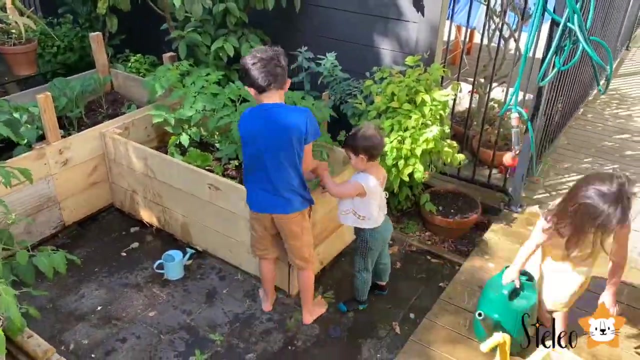 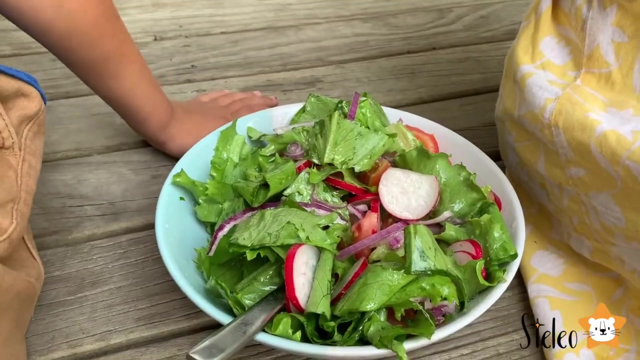 Yeah, because we have too much lettuce to only make a salad. Even radish is too much. Even radish is too much. Let's get some more. Wow, sure, My turn, Oh, sorry, My turn. So our salad is ready, isn't it? Yeah?